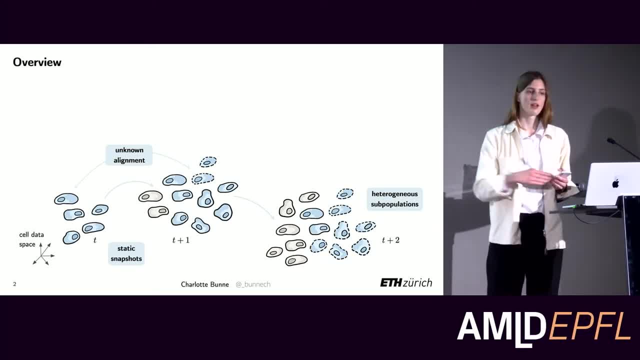 successively. do these genes change right? the trends, like the, the transcriptomic profile of these cells change over time. so we want to recover these single cell trajectories over time. so we need to find the alignment between them and, last but not least, of course, we have no clue on how. 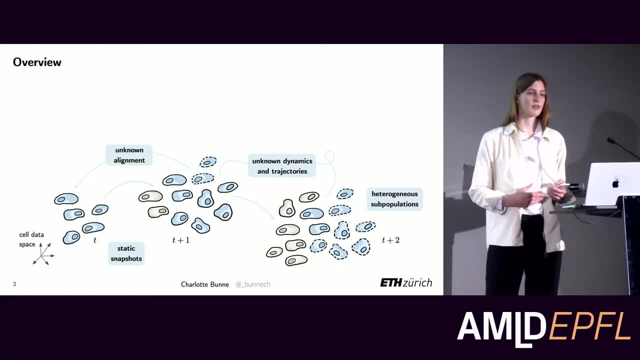 these dynamics actually govern these processes. we do not have access to trajectories at all, and these processes are highly non-machovian, so it's not enough to just look at the previous experiment to actually make predictions. we need to encounter the entire history in order to make. 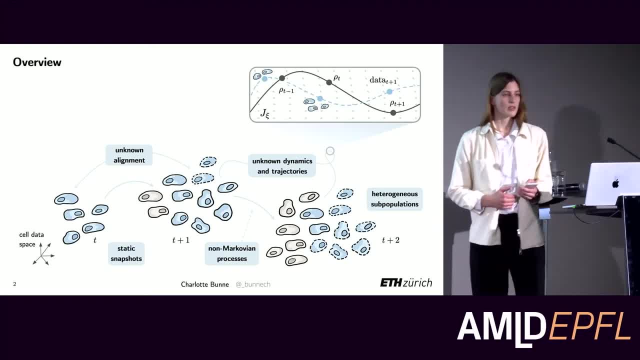 solid and robust predictions, and so this is the first thing we look at. this is part one of my talk where we try to understand- okay, so can we learn this potential on which our cells actually evolve over time in order to make predictions, and so we need to find the alignment between these cells. 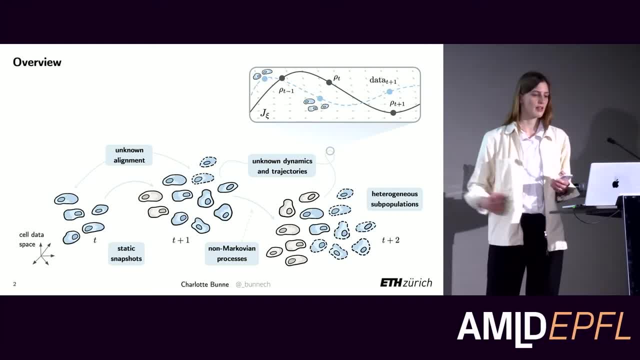 to really recover these single cell trajectories, and so this is work called jko net, something i presented just yesterday at ai stats 2022, and this is going to be the first part of the talk. in the second part of the talk, we look at a very particular problem now: the evolution of our cells. 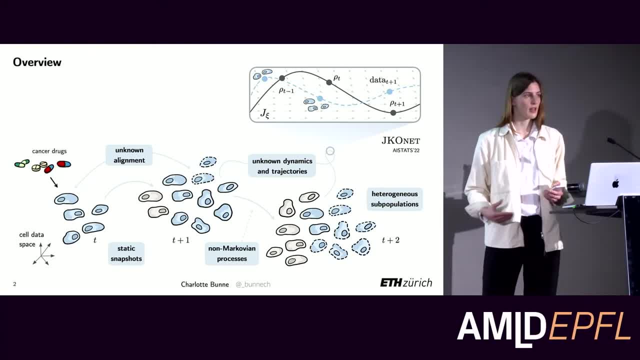 is initiated by the application of some perturbation. this can be a cancer drug, this can be any somehow outside factor. and now we are only interested in, in understanding how do these cells evolve over time and how do we learn from them? and how do we learn from them? 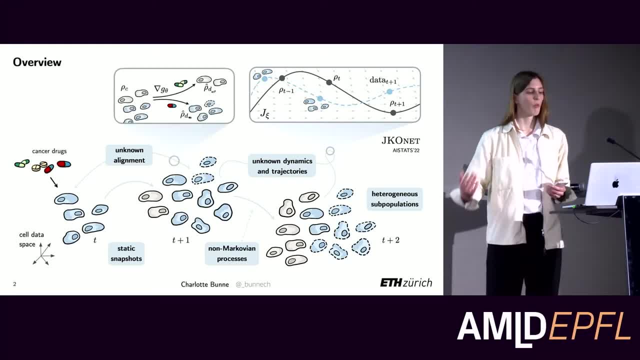 these cells change over time, so we want to understand this like one step in time. how is our population of control cells changing into the perturbed cell state? so this is a work called cellot and is currently in submission. so here we have only this one step procedure. this will be the 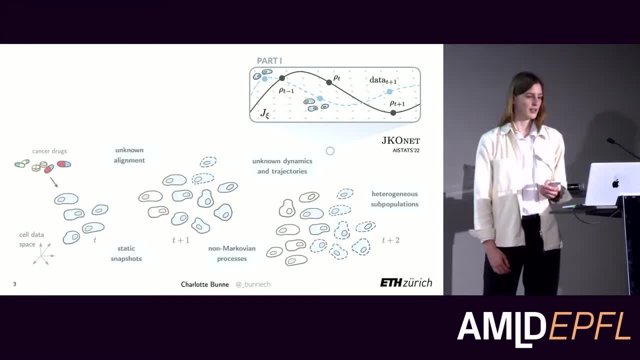 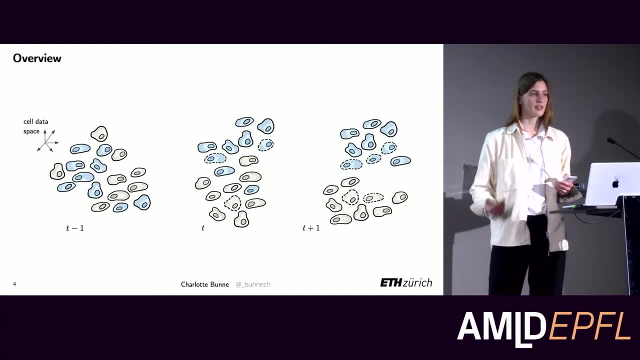 second part of the talk, so let's start with part two and let's revisit once the assumption we make on this process. so we measure at snapshots a single cell population which lies in a potentially very high dimensional cell data space and we assume that these cells evolve over time and we want to recover this evolution and this evolution might be initialized. 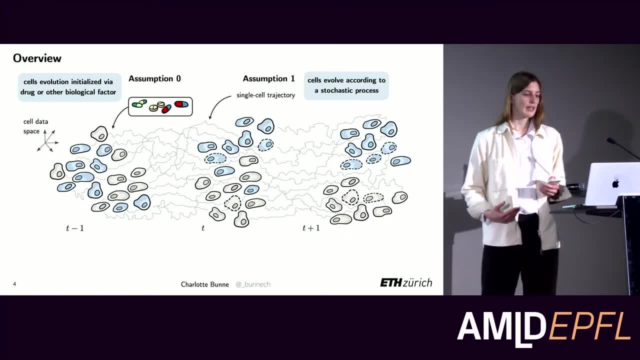 by a biological factor, a drug or whatsoever, and we assume that through our time right, this transcriptomic profile of these cells changes, or the translational profiles, or whatever molecular profile. so in this space, in this very high dimensional space, the cells somehow evolve according to our function and we want to recover this evolution. and we want to recover this evolution. 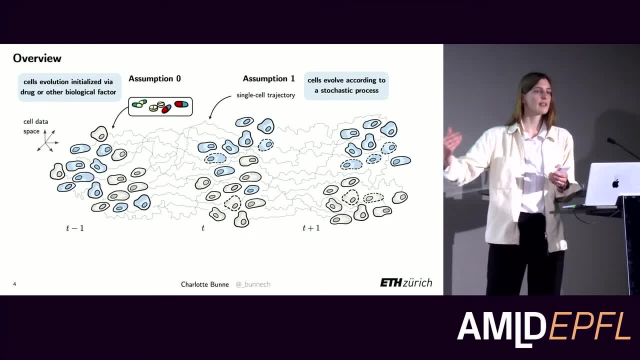 to a stochastic process. so success, like incrementally these genes change, and this is also the last hypothesis we make- is that these cells do not drastically change. it's not that like a small cell becomes suddenly star-shaped, but like it becomes slowly star-shaped. so we can actually 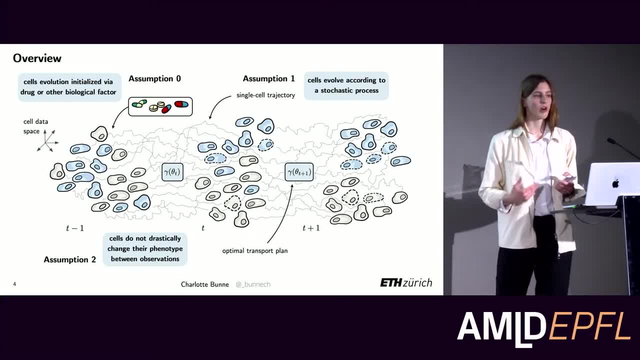 locally approximate this by something which is called an optimal transport plan, but more on this later. so we assume that we can match or align these cells in order to recover these single cell trajectories by finding the best aligned population according to this minimal effort principle, like only like a small change so that we can find the optimal alignment. 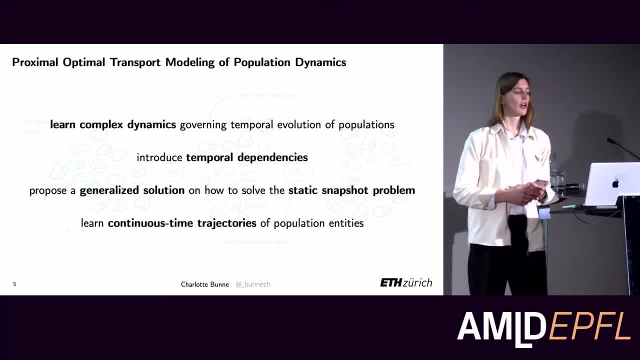 so what's the goal? in the first part? we want to learn the complex dynamics which govern the temporal evolution of populations. this can be generally any kind of population. the method is very general, it's just. our focus here was single cell data. we want to introduce temporal dependencies. 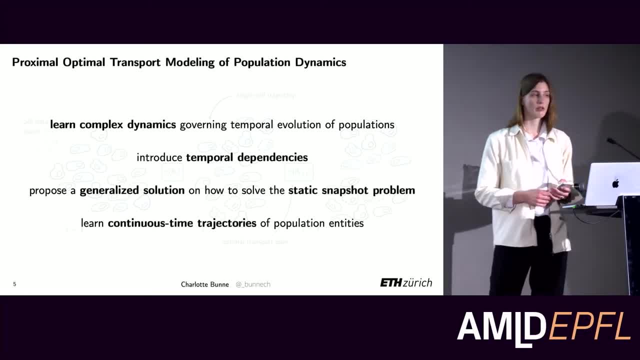 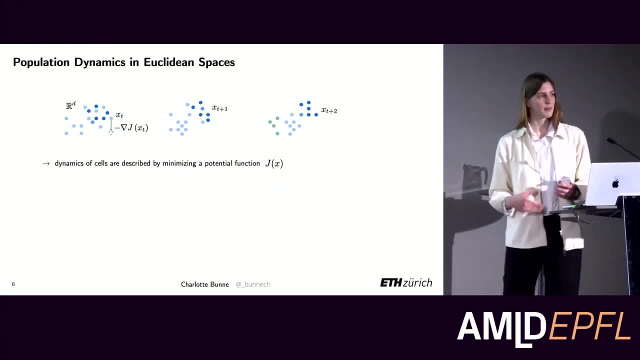 we want to learn a generalized solution on how to solve the static snapshot problem. you and learn continuous time trajectories of population entities. so let's start very simple. we have population dynamics evolving in a euclidean space. so, just like here, every cell is a vector. and now a very common assumption people make is that we can describe the evolution of 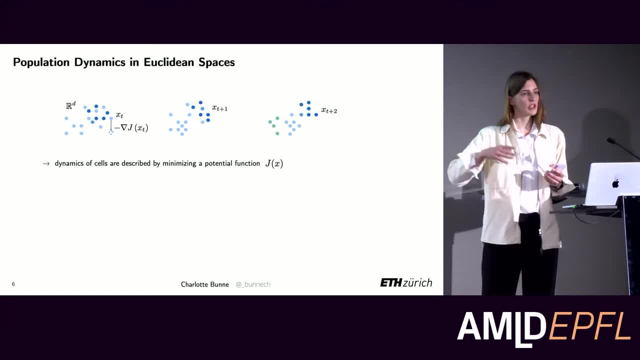 this population by saying this population over time minimizes a potential function j. that's the hypothesis, and a very common approach then is to say: okay, so let's assume that we follow the gradient direction of this potential, so the next vector at the next time step is just given by following the gradient. 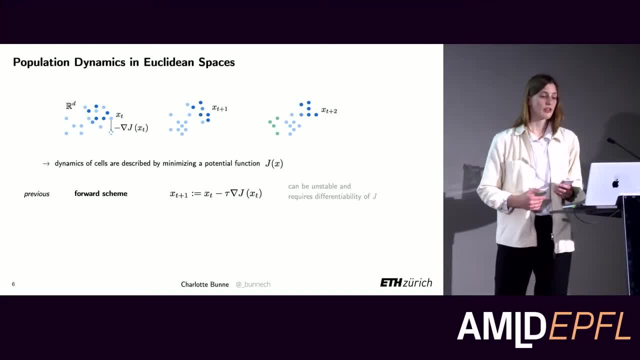 negative gradient direction of our potential function j. the problem here- and this is something we see later in the experiments- it's rather unstable. gradient descent is known to, to, to get stuck in local minima and we have certain properties. we is, we need to, our potential function j needs to satisfy. so in this work we, we propose to look at the this, the corresponding 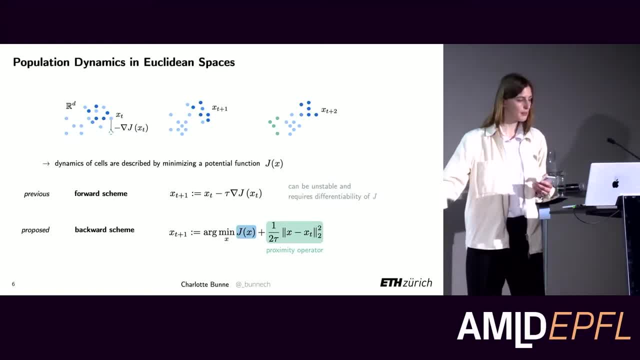 backward problem. so now the population at the next time point t plus one is given by an argument: problem over the space of all possible. next vectors x, which minimizes the energy but at the same time also stays close in space to the previous point. so this is this proximity operator in euclidean space. this is of course the euclidean. 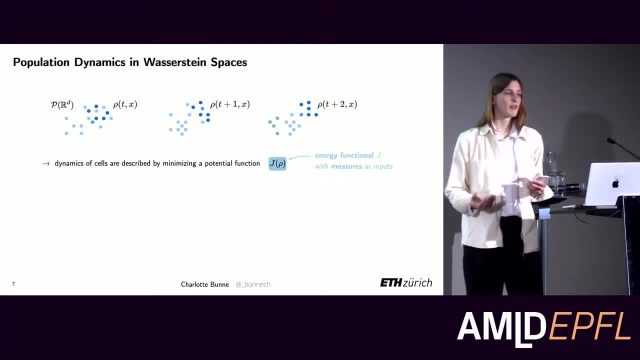 distance. now, of course, we we already as, as said, we don't have trajectories, we are not in a euclidean space. we are required to look at the population level right as we have no, no alignment. so we need to have a potential function now, taking a measure like a population as input. 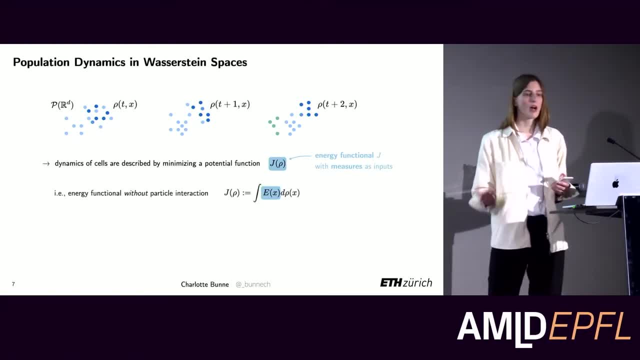 and we make also one more simplifying assumption, that for now our potential is just like the sum over all individual energies of each particle in the population. we do not consider for now any interaction, and so again we can look at the the corresponding forward scheme which has the same. 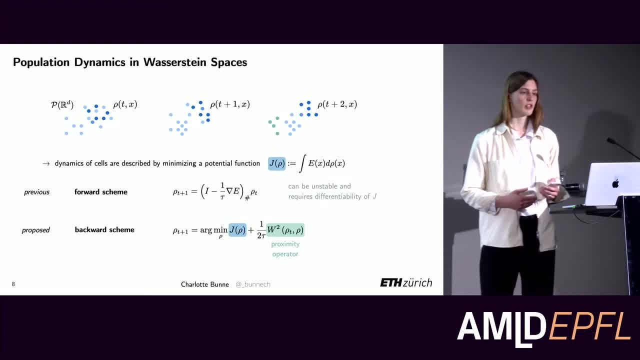 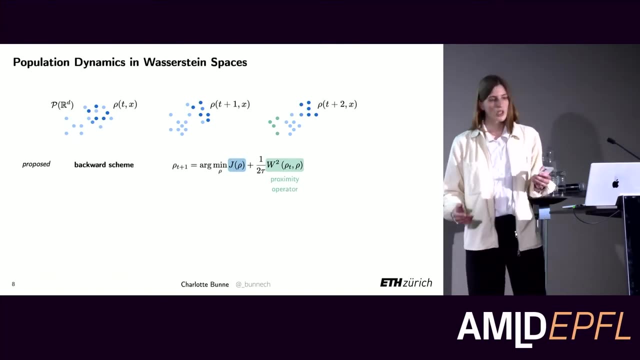 somehow pitfalls and the corresponding backward scheme, which is now an argument problem over the energy. right, we want to minimize the energy and we want to minimize the energy and we want to minimize the energy but also stay close to the previous population. now, taking the respective metric in the space of measures, being the Wasserstein distance, and just a quick reminder, 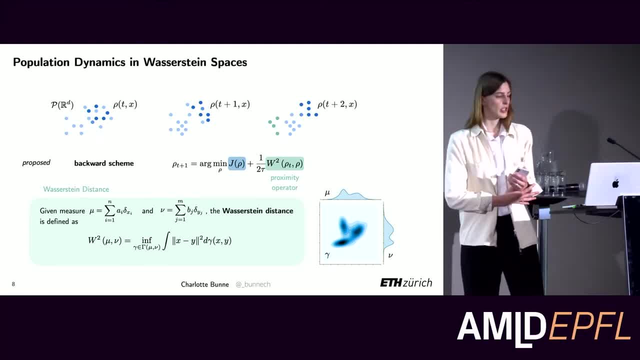 this might be a bit a lot of information at once, but just the Wasserstein distance is a distance defined between two measures, mu and nu, which is defined on this principle of optimal transport. so we want to find the transportation plan gamma which maps like mu measure mu onto measure nu. 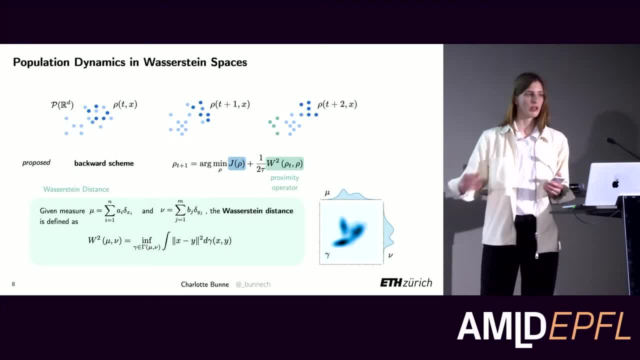 in an optimal way, meaning that the overall cost here, measured by the euclidean distance inside the integral, is like: we find the mapping such that the overall cost is minimal, and this fits. this gets us back to our assumption that we say: we find an optimal alignment such that we can best. 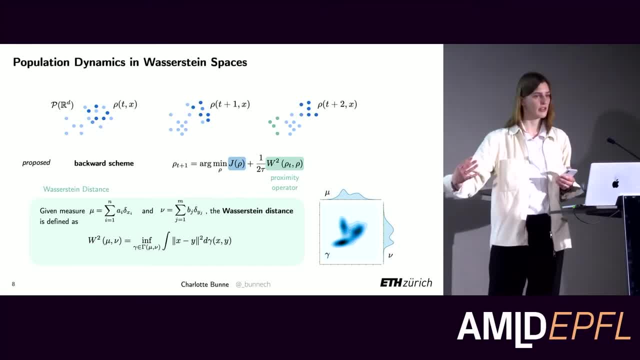 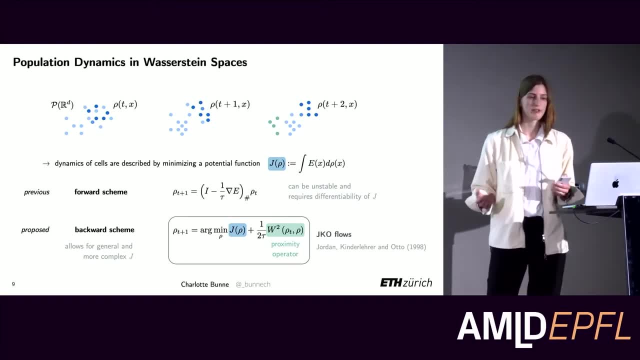 describe the incremental changes of our population in time. this is actually a very famous scheme. so this is the so-called jko flow. this proximal scheme, this backward scheme, which is um, was published by jordan kinder lehrer and otto in 1998, and so here we applied the first. 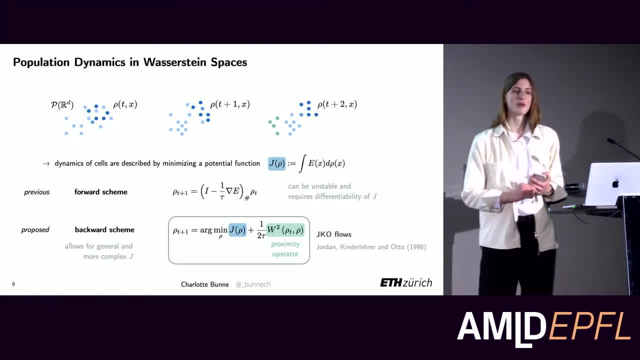 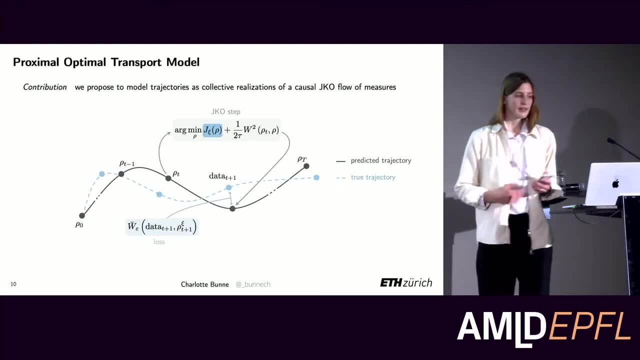 time to population dynamics. it's a famous result and it's actually the most downloaded papers of all time of the siam journal of applied mathematics. so here's our first contribution. so we model these population trajectories as a causal jko flow of measures. so, starting with an initial measure, row, 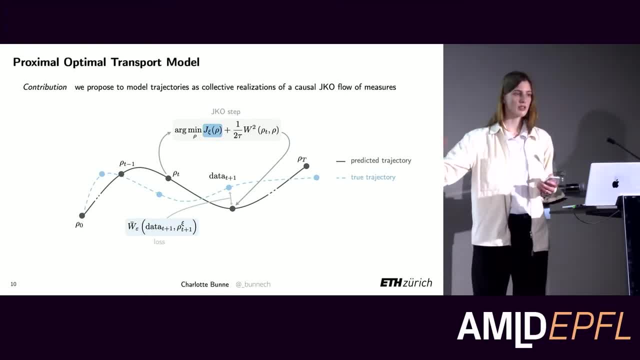 zero. we propose that the next population, the next snapshot, can be predicted by solving a jko step, where we need to, of course, learn the energy j, because j is unknown to us. so we parameterize j by a neural network and so now, at each point in time we can, we can measure how well do our predictions actually align with? 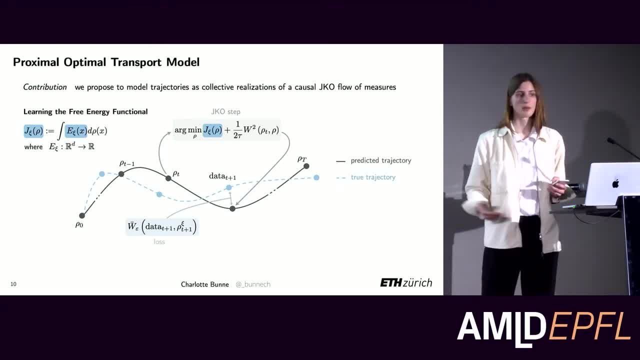 the data, the observations we have, by taking the corresponding metric, the wasserstein metric, and measuring how accurate our predictions are. then we back prop through this jko step in order to update the of our energy. but here comes the second problem. first of all, we need to back prop through an 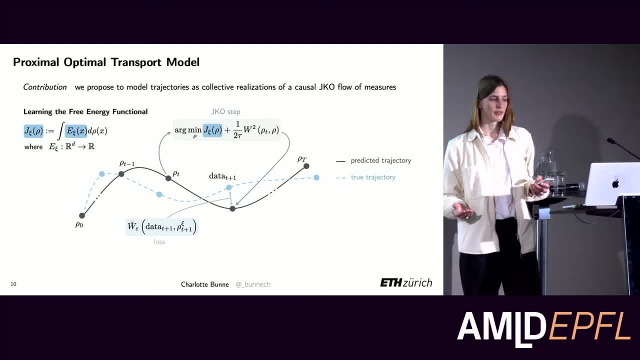 argument problem right. so that's very complicated and non-trivial. the second problem is we actually have no clue on how to solve this argument problem in the first place. it's a very complicated optimization problem over the space of all measures. we don't know how to do this, and so 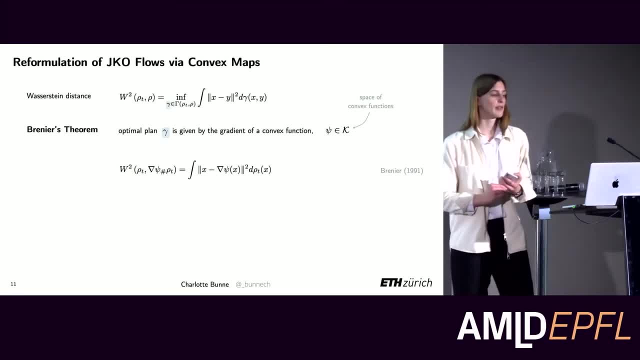 here comes our second contribution. we derive a reformulation of the jko flows in terms of convex maps and there's a very famous result in which is called the brenier's theorem from published in 1991, which states- and this is just like for now we can just take this as a fact- that the optimal transport plant gamma right, which maps. 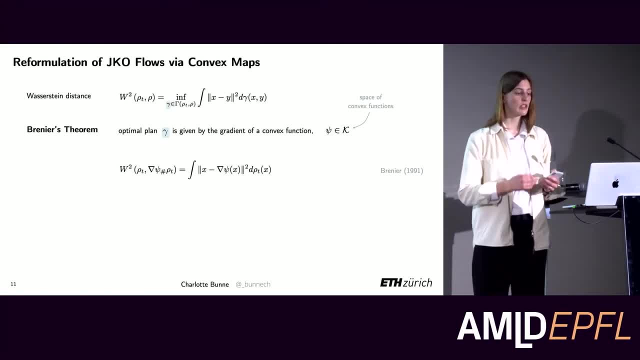 our two measures onto each other, which gives us the alignment is just given by the gradient of a convex function. so now we have a reformulated version of the wasserstein distance and also a reformulated version of the objective, and now, instead of having an argument problem over the 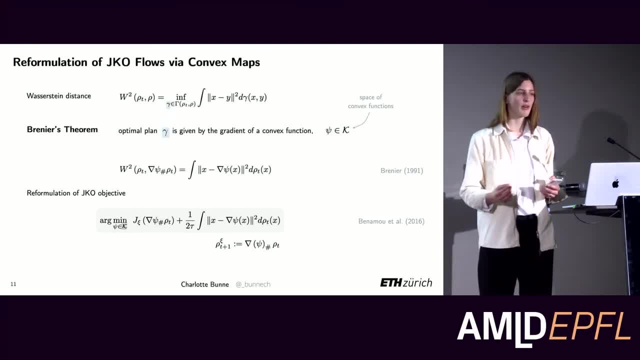 space of all measures. we have an argument problem where we just need to find the best convex function And then the next population- rho t plus one is given by the gradient of this convex function- push forward the previous population. So here we wonder: okay, how can 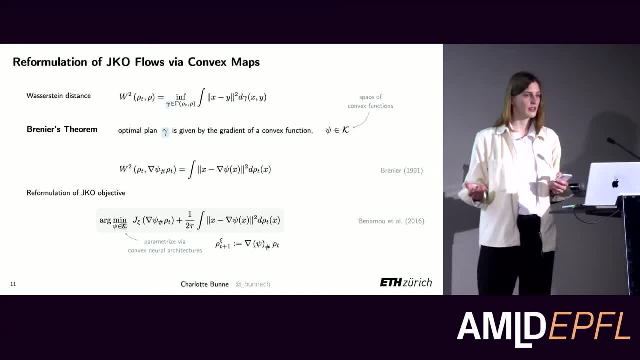 we actually? why is it easier to parametrize the space of all convex functions rather than the space of all measures? It's because we can approximate the space by just convex neural network architectures. So these are neural networks which are input, convex, so convex. 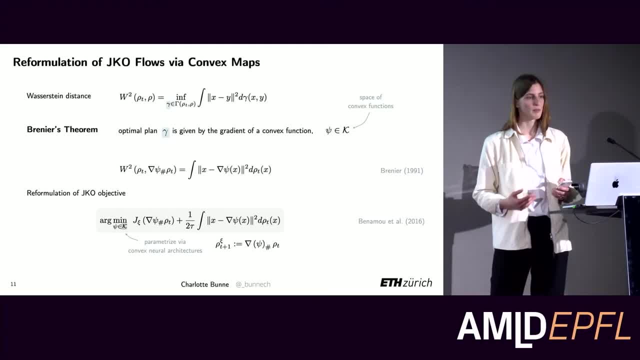 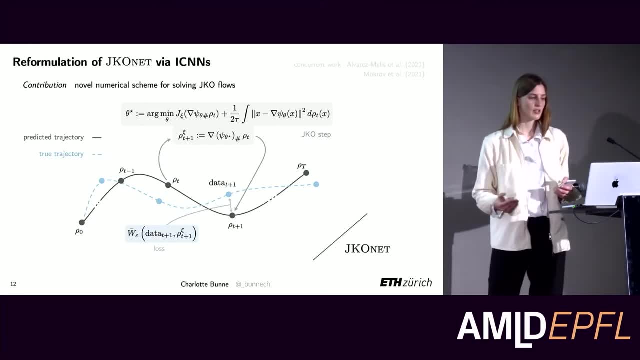 with respect to its input, And so this is an architecture proposed by Brandon Amos in 2017.. So now here we arrive at our final GKO net. So we say, okay, we can learn the population dynamics by predicting the population. at the next step, by solving a GKO. step Here our reformulated GKO. 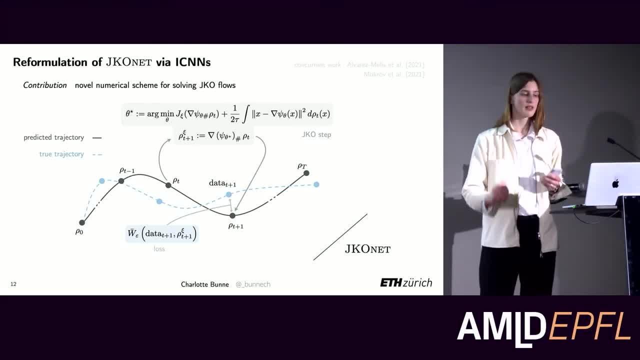 step which actually requires us to find the optimal convex function And then the population. at the next time step, rho, t plus one is just given by the optimal version, so the one we found after successive minimization steps of this GKO objective. 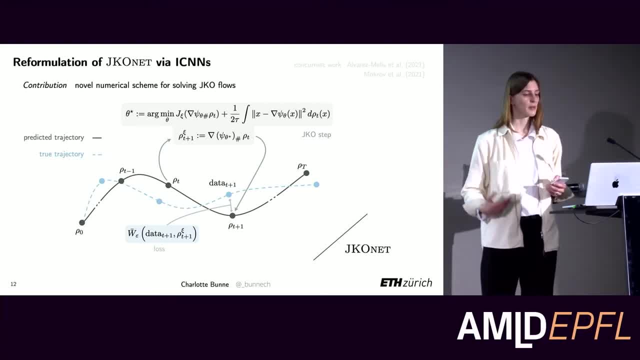 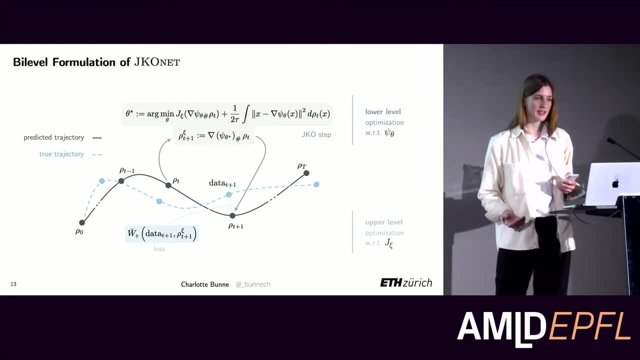 So this optimal convex map gradient of this optimal convex map push forward the previous population. So what we see here is that this is actually a rather complicated bi-level optimization problem, because our primal goal right is to learn the energy function on the top, on the upper. 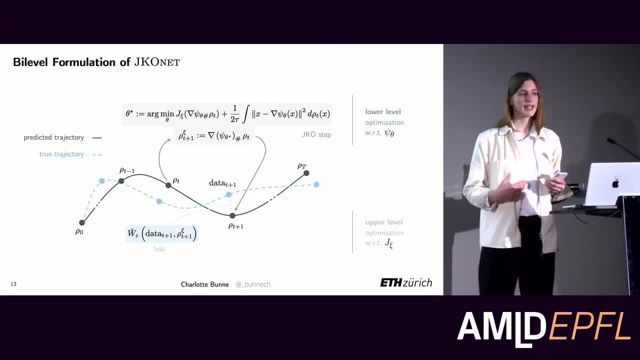 level And we can see that it's recurrent. So we can learn the energy function on the top, on the lower level, And we can see that it's required to have an insight, like a nested optimization problem, on the lower level, where we need to find the optimal convex map. And the next challenge is 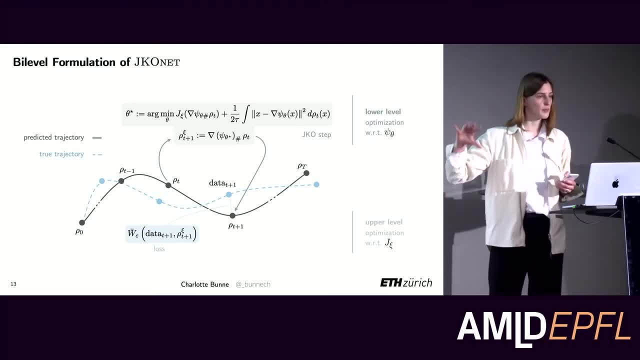 that if we look at the loss term here, the Wasserstein distance between the observations, the data and the predictions at the next time step, we realize there's actually no direct dependency on the energy function anymore. If we look at the population at the next time step. 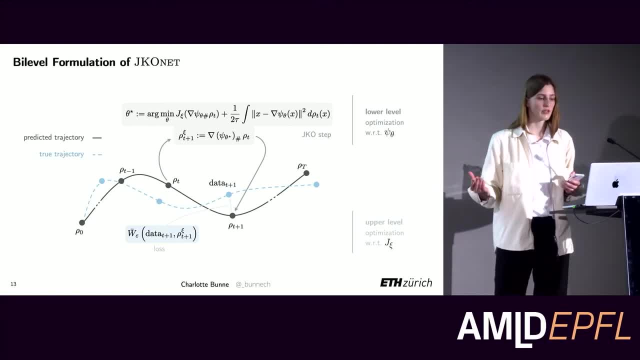 we realize this is actually just the optimal convex map Or, like convex function, push forward the previous population. So the dependency on our parameters of the energy, which we seek to learn only, is like available in the updates, in the gradient updates of our optimization of this convex map. So we have this bi-level optimization problem. 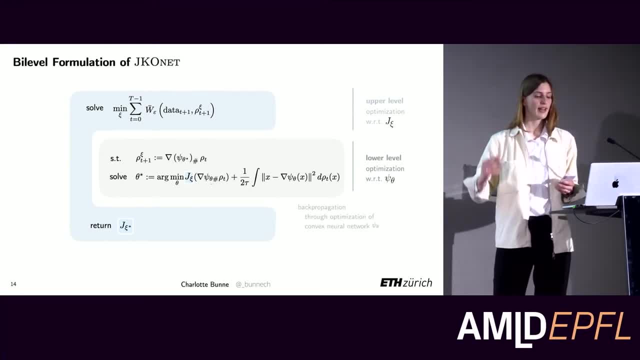 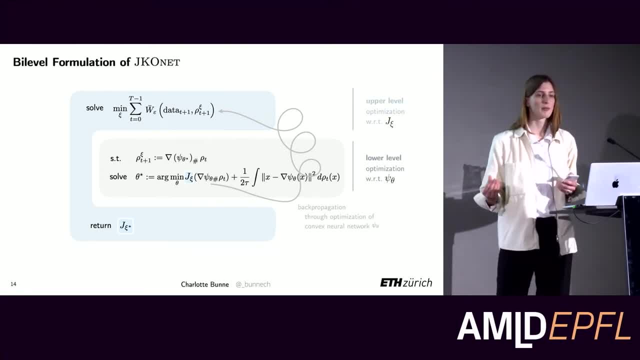 how to how to how to update the parameters, or like find the optimal parameters of our energy. We do this and we also successfully were able to put this into like a fully differentiable bi-level optimization framework, And what's interesting here is that there's actually very 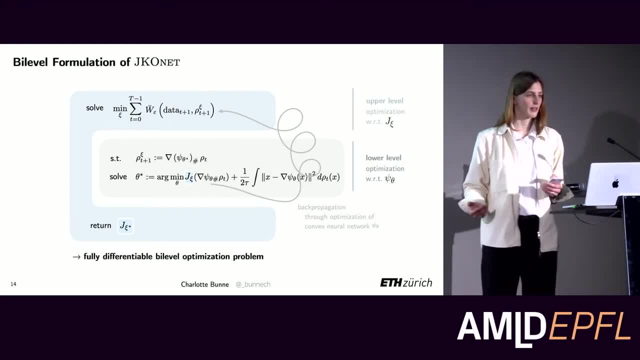 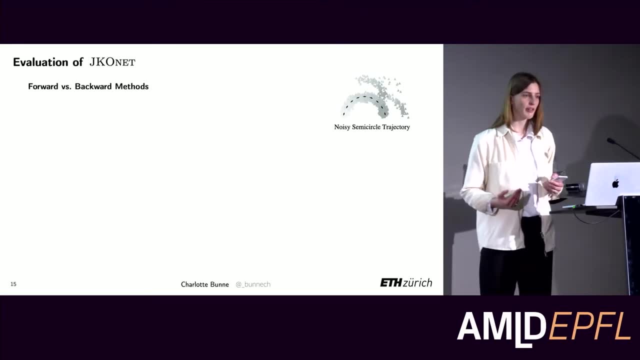 like a lot of related work or connected work in the field of meta-learning. So many shared ideas here, And so let's understand why this is much better than looking at the forward method. Here we have a very simple example where we just have a noisy semicircle trajectory. 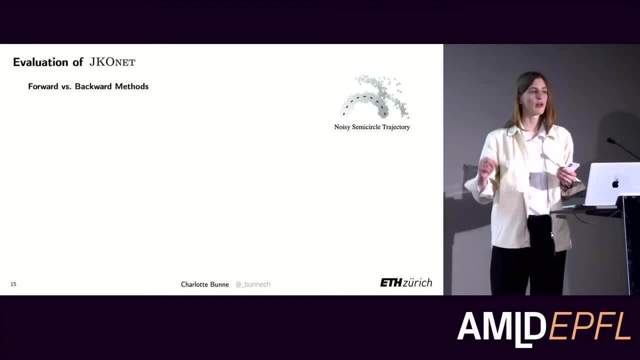 So we start on the left and the task is to just like move along a semicircle, our Gaussian blob, And then, at later time points we actually have some noise, some corruption, but every time different. But in the end, what we want to learn, 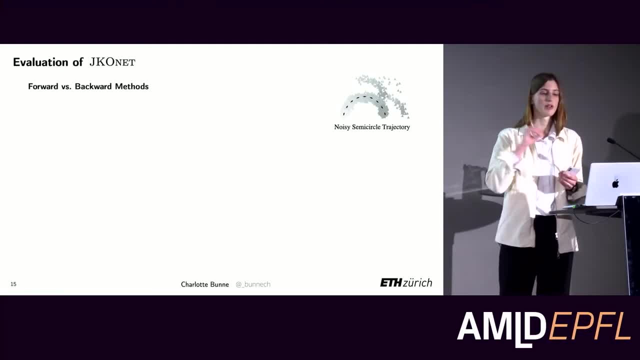 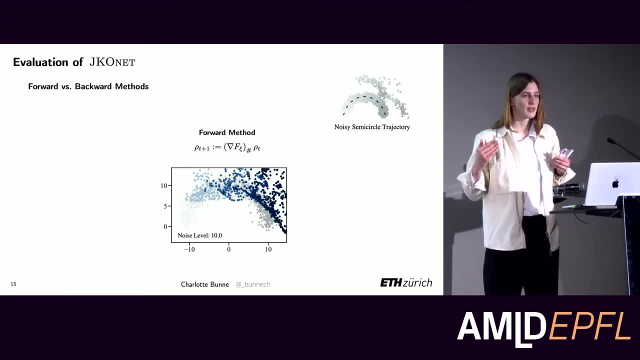 and this is also what we evaluate on. we want to learn the noisy, we want to learn the semicircle trajectory. So now the forward method just moves into the gradient direction of this potential. So the potential directly determines where we go in the next step. right? 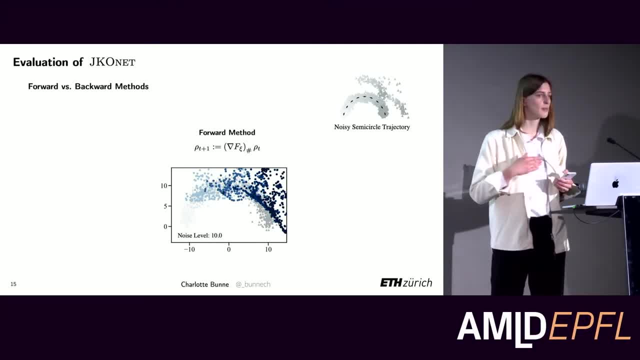 So it completely overfits the data. It just learns perfectly to mimic the level of noise in our data, While if we look at our corresponding backward scheme, we have a decoupling of learning, the energy which determines our flow and the push forward like the optimal mapping. 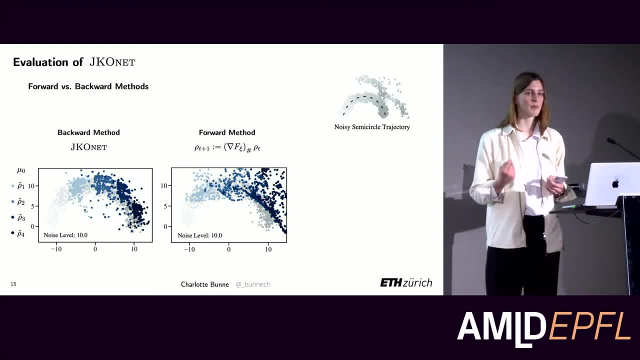 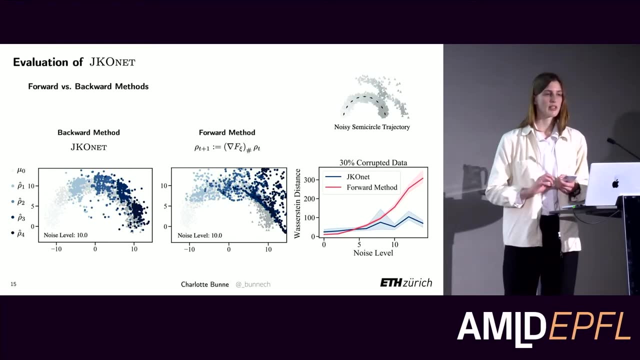 which is required to be an optimal transport. So we have here a prior right that this is supposed to move optimally and this resolves these pitfalls. the forward method. And if we look at just successively adding noise over time, the forward method really like just blows up. 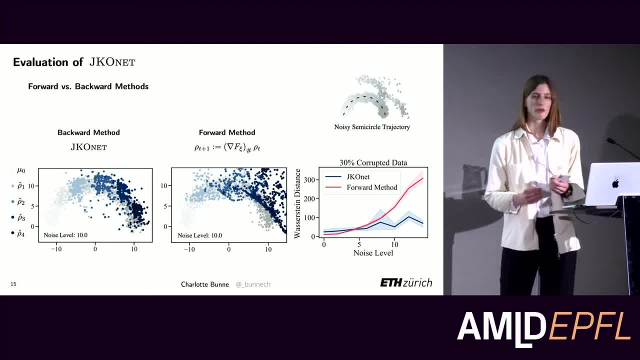 At the beginning, right where the noise level is close to zero. of course, the forward method perfectly fits the data. It just overfits the data heavily and it's even better than our method. But our method is really robust to high level of noise. 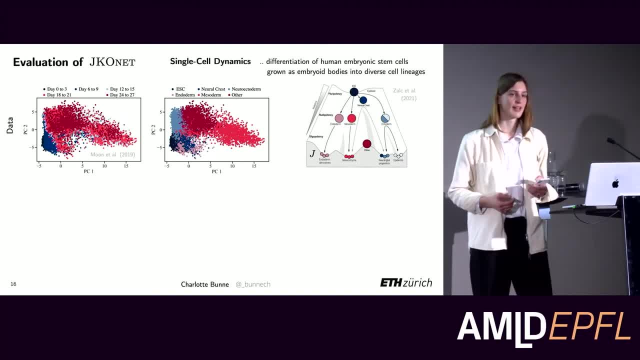 And why is this important? If we look at single cell data, of course we have high level of noise. There's a lot of experimental noise, There's biological variability and all these kind of things we need to care about. So we have a lot of experimental noise. 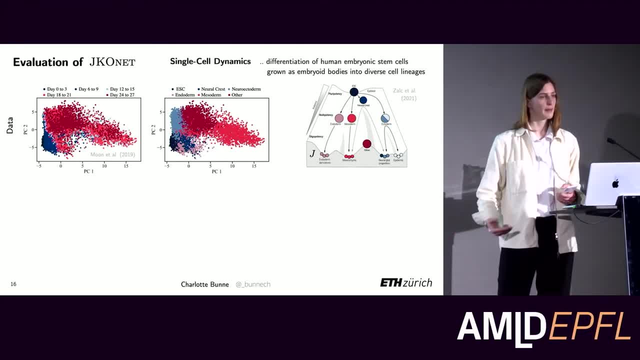 So we have a lot of experimental noise. So here we have an example where we applied our JKO net on, where we have, at the very top, embryonic stem cells which differentiate into very different branches or lineages, So mesoderm, endoderm, ectoderm. 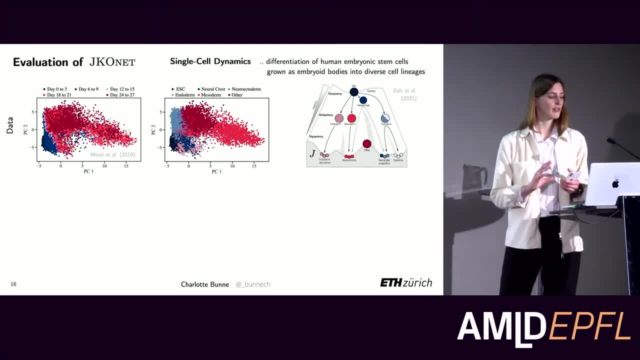 I'm myself not an expert in this, But so on the left you can see the data in the first two principal components, where we color each cell of the trained data set with the corresponding time point and in the middle with the corresponding lineage information. 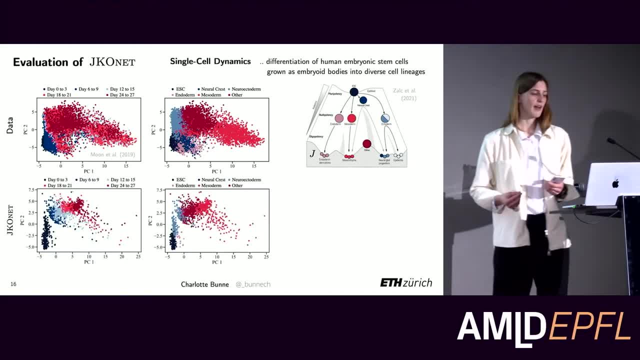 And here we have, just like, the predictions of our JKO net And we can see very well that, just looking at the first two principal components, this, like flow and time, is very well captured And we are actually able to really capture the biological heterogeneity. 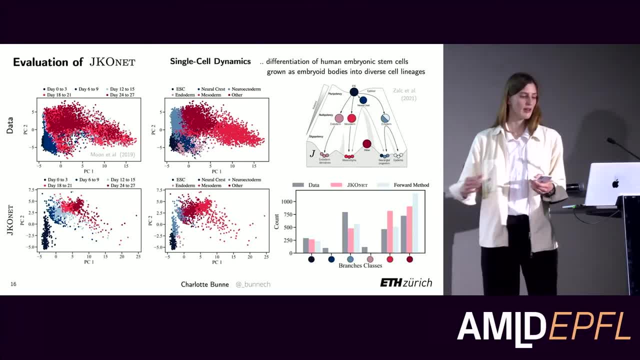 really capture all cell types. So here we can just see we have like six different branch classes, one being of course the stem cells, where the starting population, and the other five are the ones which we basically have. So we have a lot of information. 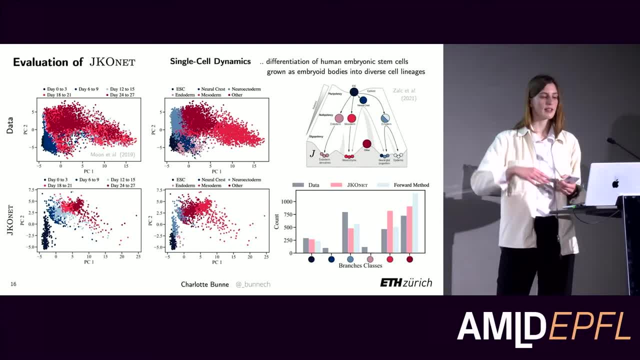 So we have a lot of information And we can see that even far away populations which only arrive at later time points are captured fairly well. So this is only visual inspections. I mean, of course, the paper. we have also this quantified in numbers. 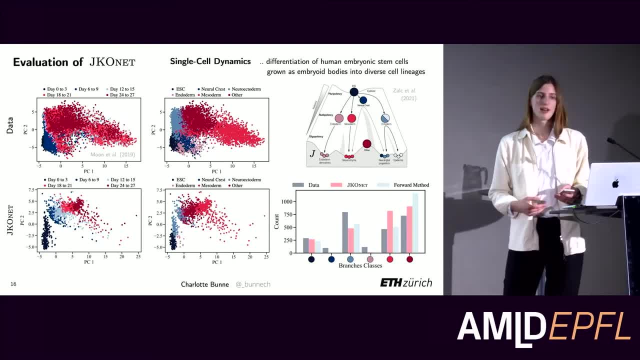 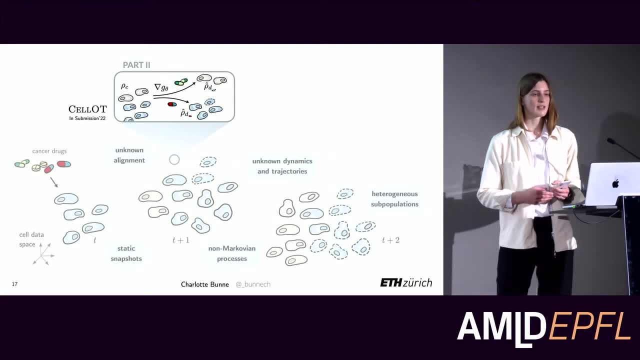 and I refer you to the paper for more details on this, But this was a very nice result. We were super happy about this, So let's look at the second part of the problem. So here, instead of actually learning the entire trajectory, 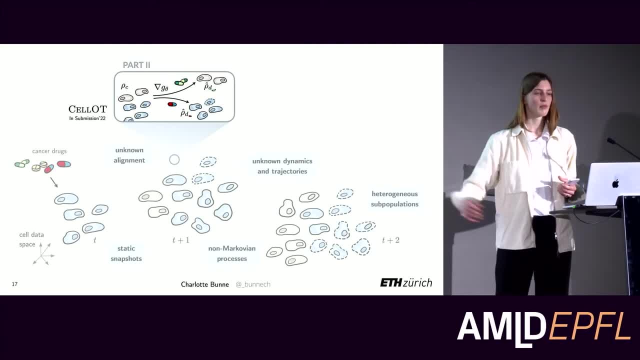 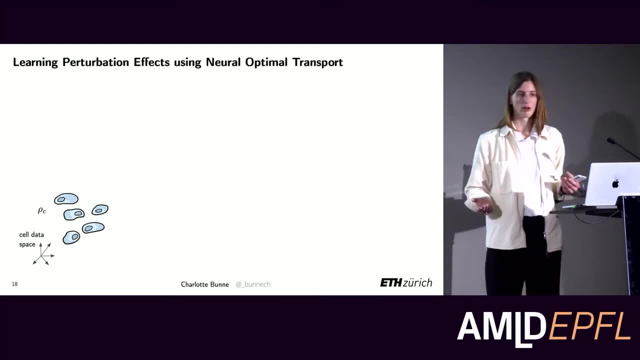 the energy which governs these processes over time. we just want to understand how does a population of control cells, before a treatment is applied of a patient, for example, changes into the perturbed state And this allows us to then understand. okay, so, given my control cells, 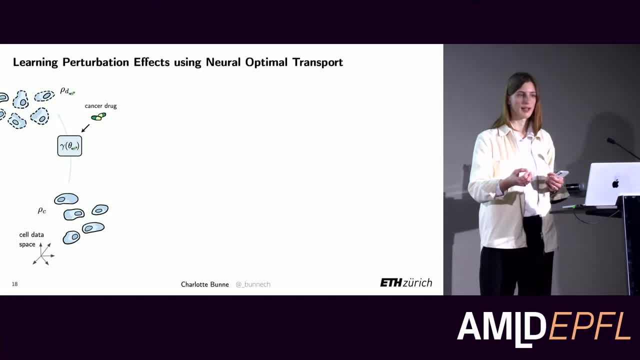 which of these cells actually are sensitive to the drug I apply, Which die right, Which are where is my drug effective, Which subpopulations are actually responsive to the drug I apply, And then we can do this. We can do this, of course, for every type of drug right. 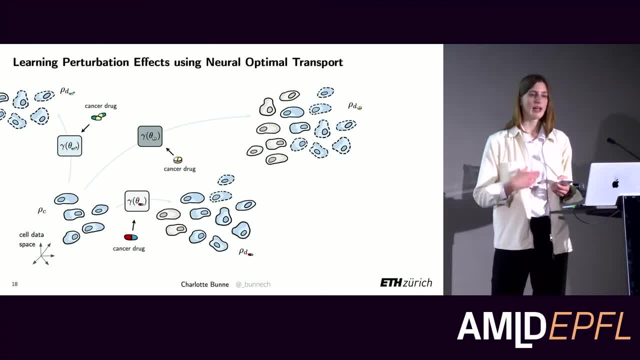 We can learn this underlying map, yeah, And predict the treatment outcome of a patient for all potential types of treatments. So the goal here is to learn the drug perturbation again via an optimal transport plan, Because the assumption is that after applying a drug to a population, 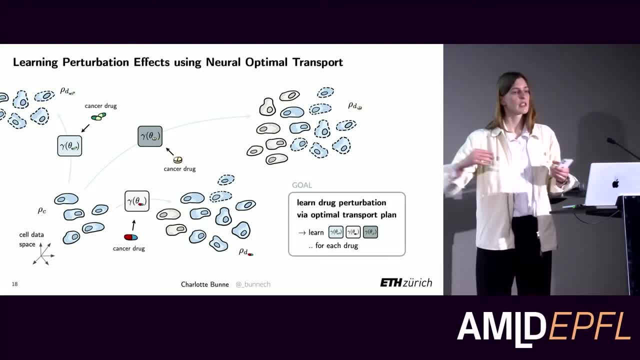 success like: incrementally right, The gene expression level of these cells is changed right, So they might be. They might become apoptotic and we see this in certain morphological features over time And we do not have rapid changes. 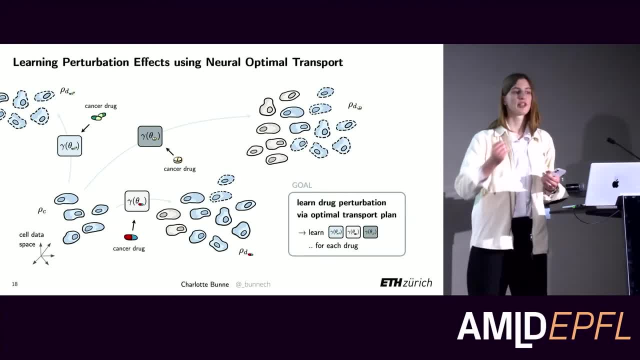 but we can find the optimal alignment by actually solving an optimal transport problem between them, Because these cells still move in the minimal effort principle inside their space, right. So how do we do this? Let's again start with the primal optimal transport plan. 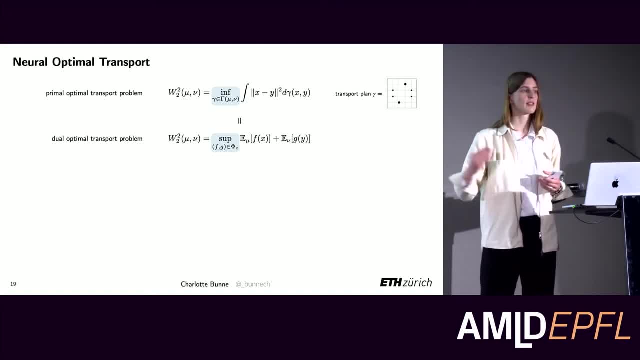 where the goal is to find the plan which minimizes the overall cost. right, So here. So here, with the L2 cost, there's a corresponding dual optimal transport problem where, instead of having minimizing over the optimal transport plan, we actually try to find an optimal pair of dual potentials, F and G. 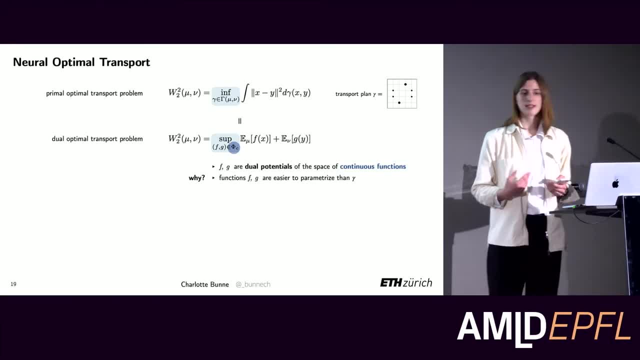 which lie in the space of continuous function. Why is it interesting to look at the dual instead of the primal? It's much easier to parametrize two functions than parametrizing this optimal transport plan gamma. So there's again something which connects. 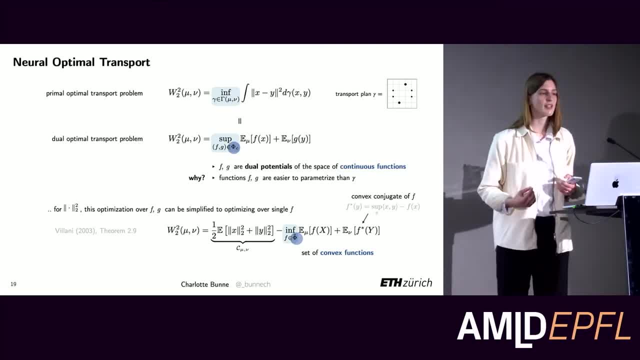 to the optimal transport plan gamma. So Brunier's theorem- and I guess you already see, given that you see the word convex function, that the principles here are applied are similar to what we have seen in the previous work. We can actually say: instead of having an optimization over F and G, 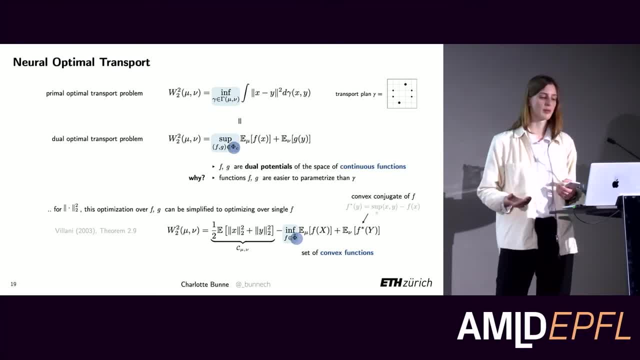 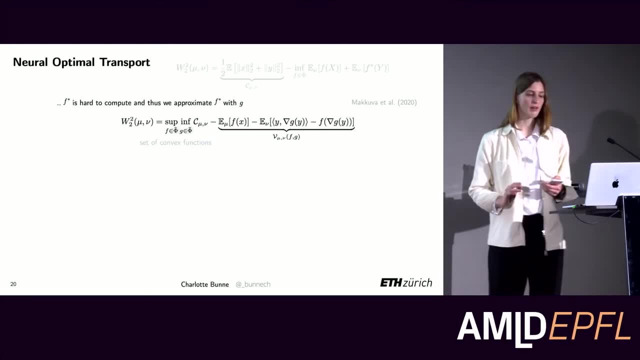 in the case, we look at the L2 cost of the optimal transport problem. we can simplify this to an optimization over a single function and its convex conjugate, And then, following results by Mark-Huwe et al, in 2020,. 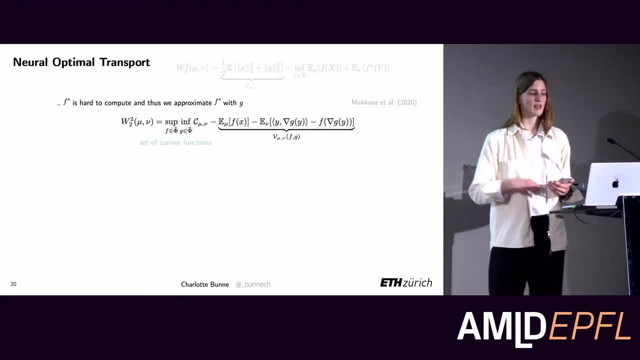 we make one approximation which says that because it's hard to approximate this convex conjugate, we just parametrize this by another convex function and now we have a min-max problem. or Mark-Huwe et al derive a min-max problem. 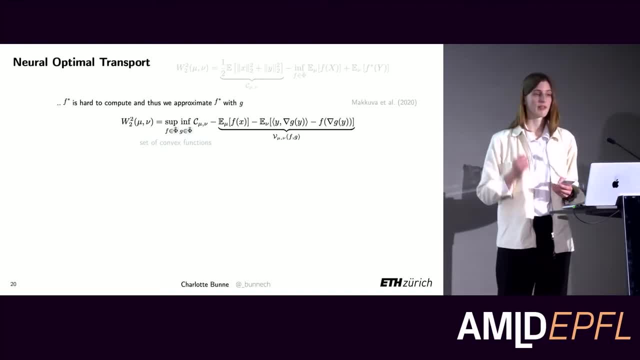 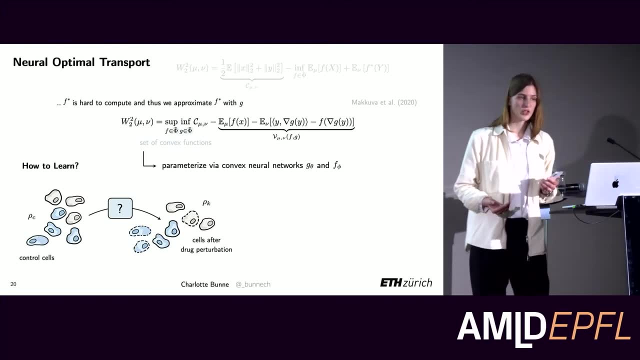 over the set of two convex functions which give us then the plan or which solve this dual optimal transport problem. So again, these convex functions, we can parametrize them by convex neural network architectures, and this is exactly what Mark-Huwe et al propose. 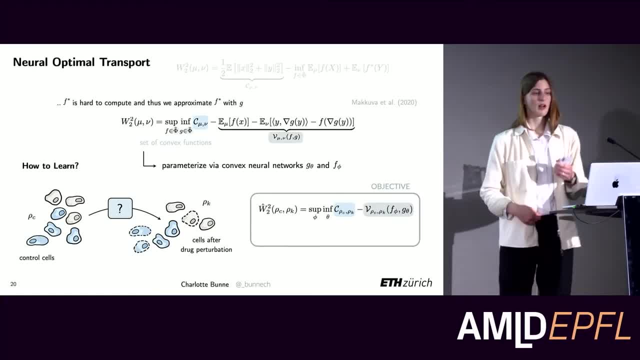 And so what we're going to do is what we do now- is that we say, okay, so we solve this in an alternating scheme, right min-max between two convex potentials, and find these parametrizations, find the optimal set of parameters. 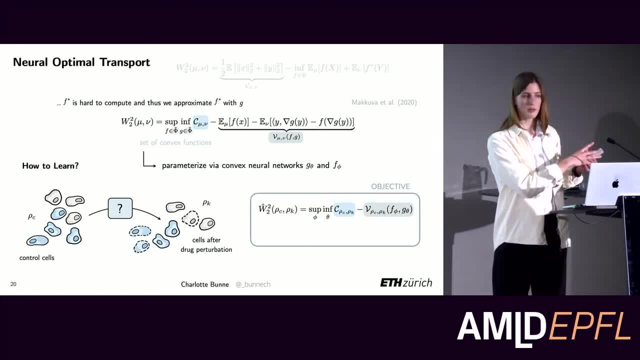 for a problem consisting of a control population and the perturbed, the corresponding perturbed population, where we don't have the alignment right, And then the optimal transport or the map, like the optimal map for each drug K, is given by the gradient of this convex function. 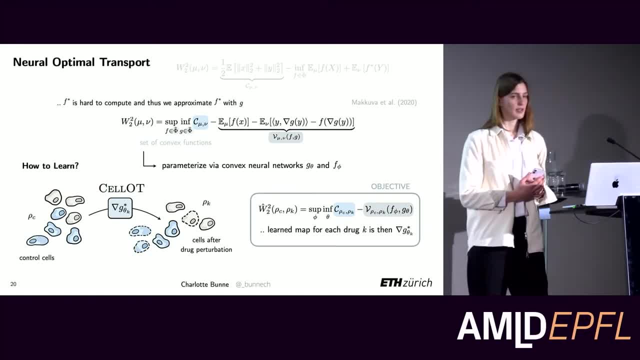 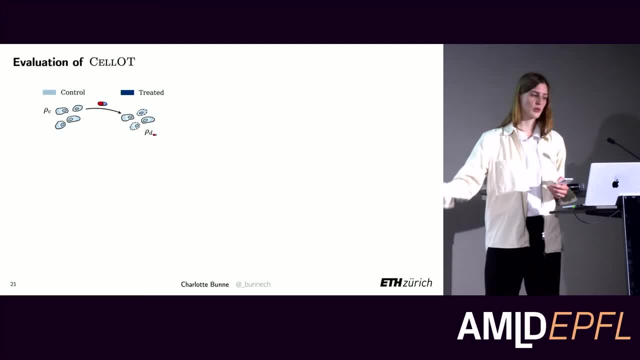 So this is something, a framework, we apply to single-cell data as well, and which we call CELOT. So now we have a control population as well as a treated population after this perturbation was applied, And what we do measure here. 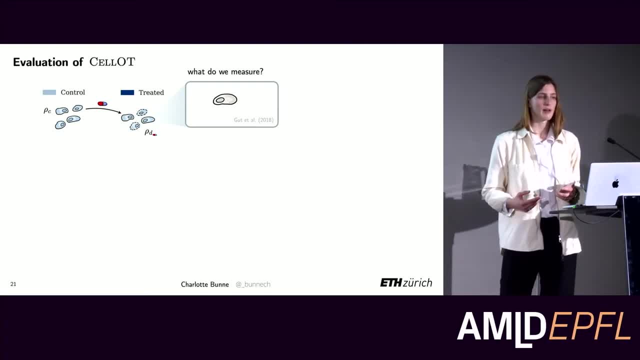 here we don't look at single-cell RNA-seq data, but at a data like a method developed by Gabriel Agut in 2018, where we have a cell and we can, under the microscope, observe certain morphological features. 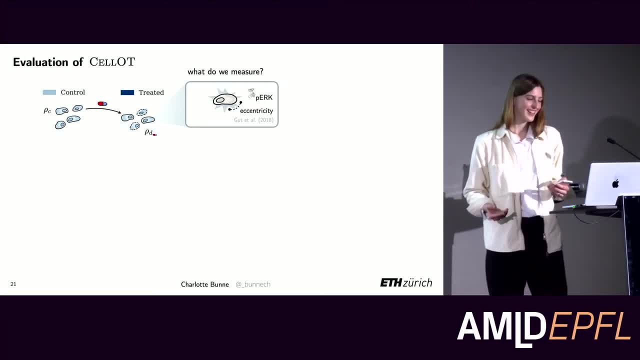 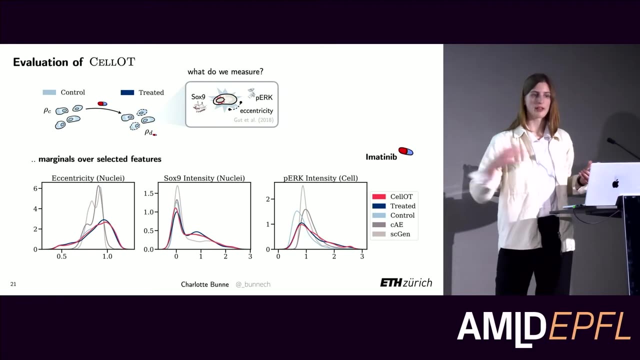 such as eccentricity, as well as certain signaling features throughout the entire cell or signaling features only present in the nucleus. So, given this, we can look at the marginals of the control and the treated population, So meaning like somehow. 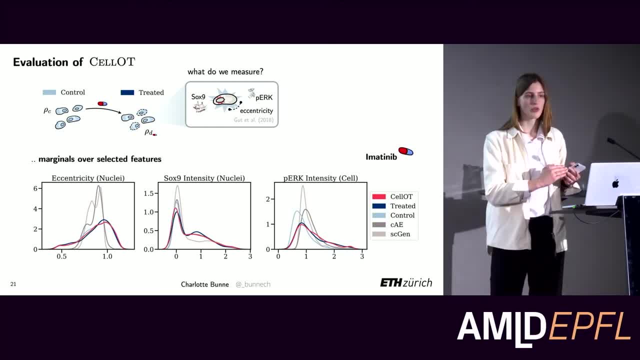 how the distribution of the presence of this feature inside my control population. this is something you see here in light blue. and then the distribution of these features in the treated population. right, We never have an alignment, but we can at least look. how is the distribution. 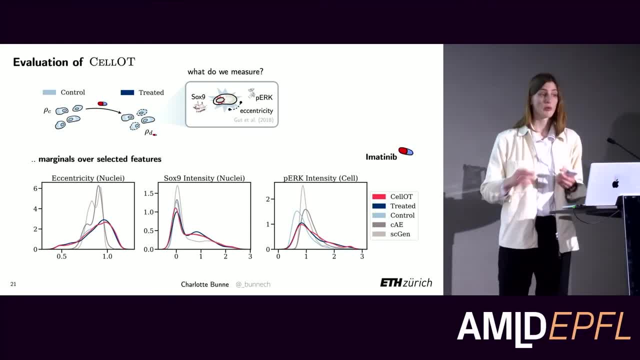 of each feature in each population. And so now we want to learn that, given the control population, moving them with our map, with our learned map, how well do we actually match this distribution of this feature in the treated population? And we compare this with two autoencoder-based methods. 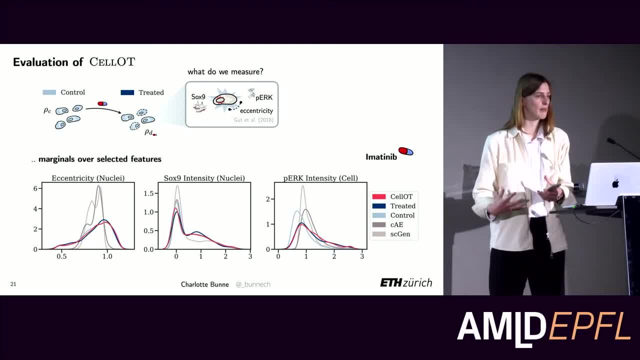 which really rely heavily on a good lower-dimensional embedding in which they can model this shift as a linear shift. in this lower-dimensional embedding, Our method by just directly operating really with this like strong modeling hypothesis, is much better in actually fitting the treated population. 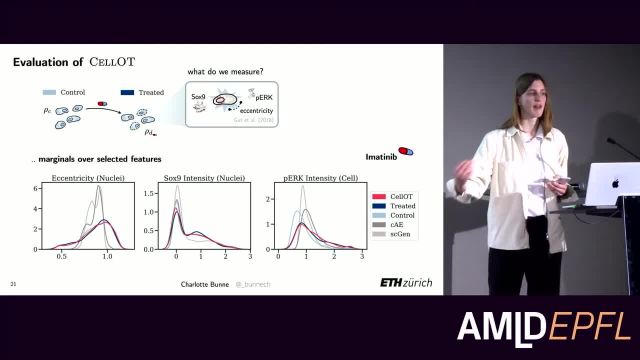 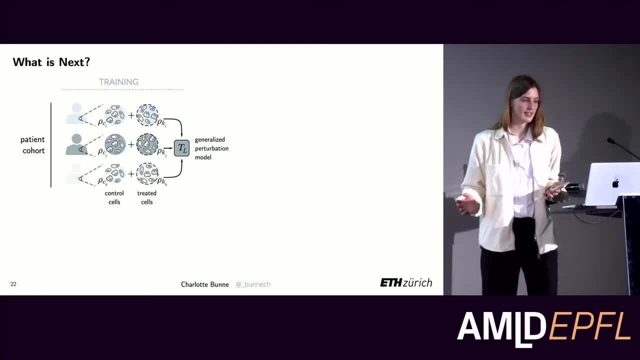 and really like matching the population observed after applying a drug, And now we can learn these maps for all drugs. So that was very great news. So what's the next step? So- and this is something we are currently on- 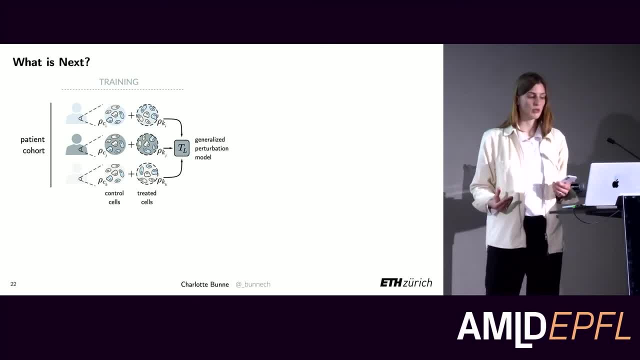 and we can just learn a generalized perturbation model over a set of patients where we capture somehow patient-specific effects but various patients, with the hope that then in the clinic, when we have a new incoming patient, we can take this trained or learned perturbation model. 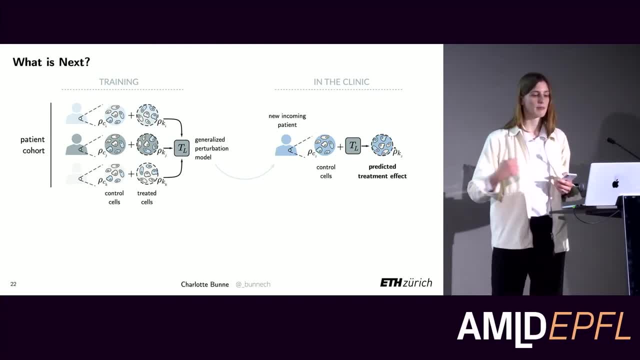 and apply this to the cells we can take from this patient and predict the treatment outcome of this. So what is the challenge here? Of course, on the one hand, we want to learn a very coherent and robust perturbation model, right. 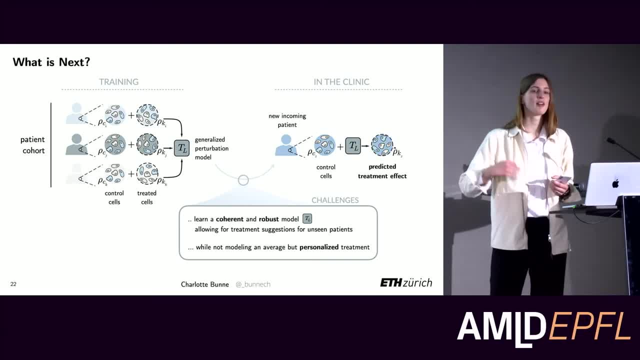 But at the same time, right, we don't only want to model a population's average, right, We want to really like capture a personalized treatment strategy for this patient. So this is the big challenge in this part. So what have we talked about, right? 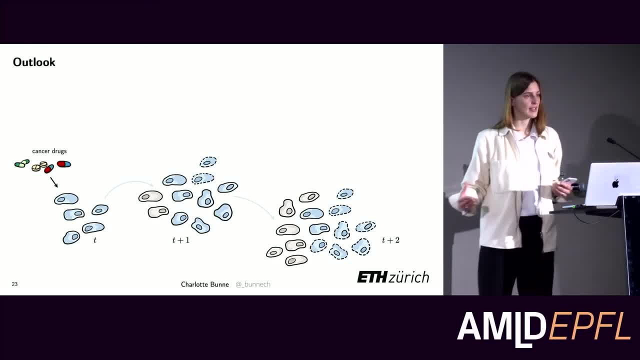 Like, of course, for drug discovery, or just like a general understanding of developmental processes in cells, or like in humans, it's very important to understand the evolution of a cell population over time. how do transcriptomic translation profiles change over time? 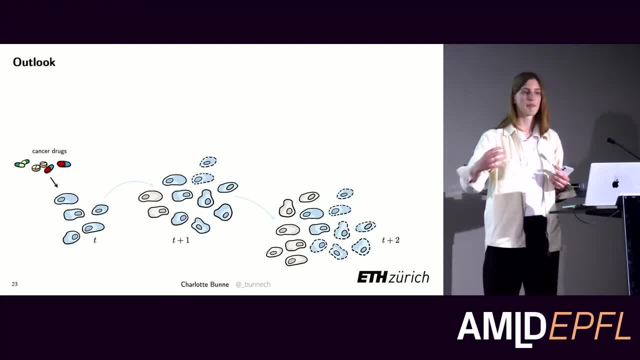 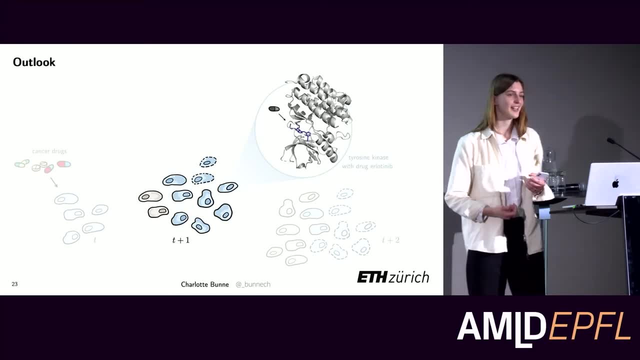 and how can we learn either the potential or just this like map which maps us into the perturbed state? But of course for drug development it's very important to really look inside a cell right Like really understand what happens on the molecular level. 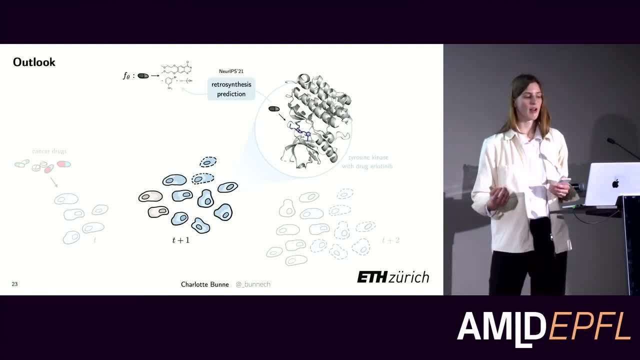 And this is some previous work of mine which has focused on retrosynthesis predictions. So, given a drug, how can we actually recover the synthones, which helps us then to find like synthesis plans for these drugs. This was presented last year at NeurIPS. 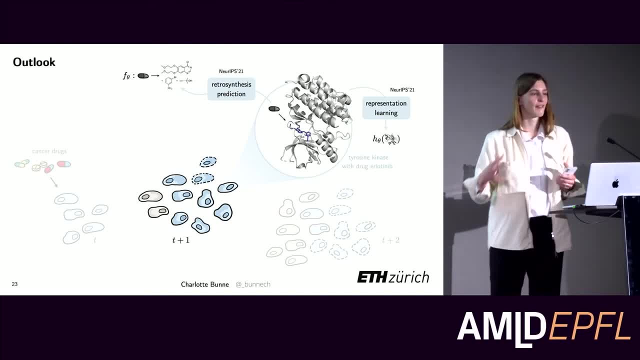 Then other work of mine has focused on given a very complicated protein right which is always part of each signaling cascade or whatever part of the process. how can we actually do machine learning on these super complicated objects? They are not only a sequence. 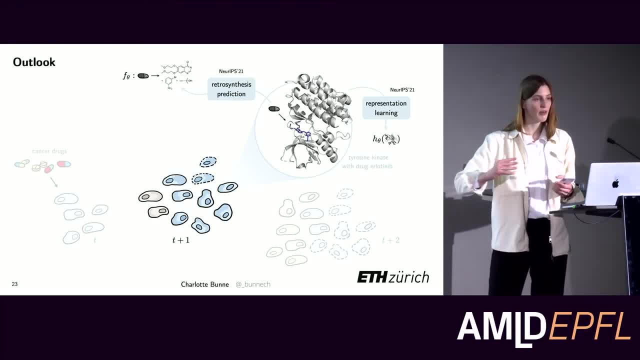 they also have a very complicated structure, a very complicated surface, which is crucial when we look at the binding. And so here we developed a representation learning algorithm which allows us to somehow use these objects or like do machine learning. 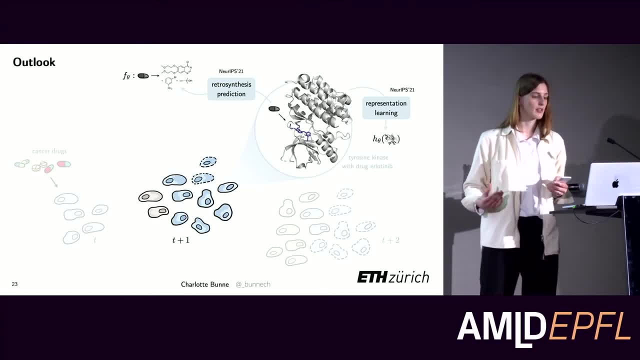 on these very complicated macromolecules. And the last work of mine which I want to feature is concerned with rigid docking for proteins, also crucial for protein or like for drug design, where we want to understand: okay, so somehow, how has a drug an influence? 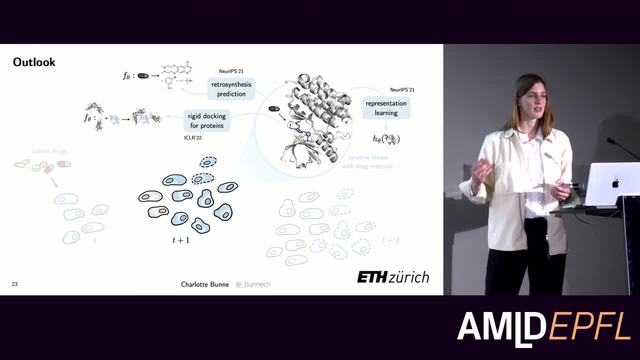 on the underlying rigid protein docking, Like how well can a protein still bind? And this is also, as the other two methods, based on the principles of geometric deep learning, and I think later in this workshop we will hear a lot about these kind of works. 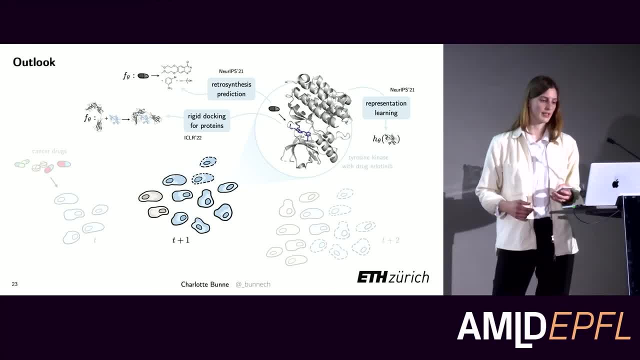 This is going to be presented this year at ICLR in a couple of weeks And with this I want to also thank the NCCR Catalysis Grant for funding most of this research presented in this work and for supporting my PhD throughout the years. 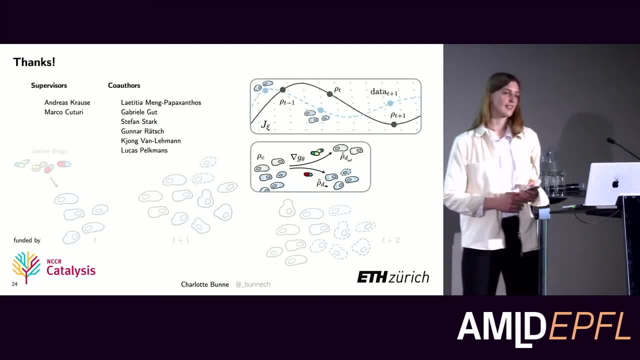 And I want to, of course, thank my great supervisors, Andreas Krauser and Marco Coturi, as well as all my co-authors which have made these works possible, which are Letizia Gabriele, Stefan Gunnar. 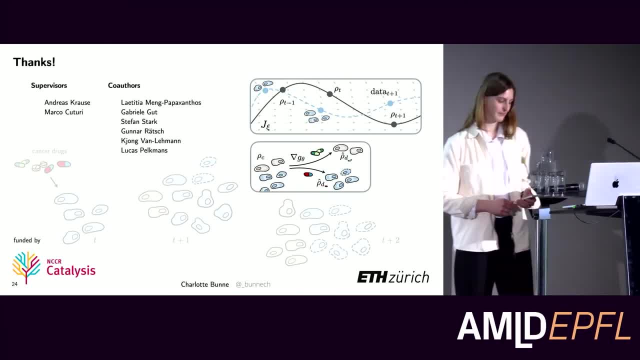 Kyung and Lucas. So thanks. Thank you very much for the great presentation. Are there questions? I have one, So just one microphone. Where's the other one? Okay, Hi there, My name is Adam. Thank you for this work. 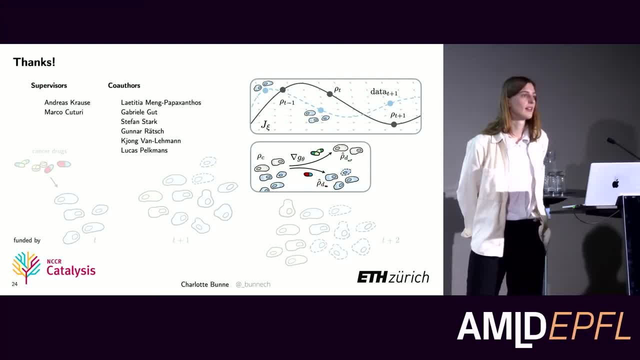 It's really elegant work and this is a theory that really lies close to my heart. I just want to understand a little bit, kind of what your theory is capable of and some of the limitations. So I'm a mathematician. 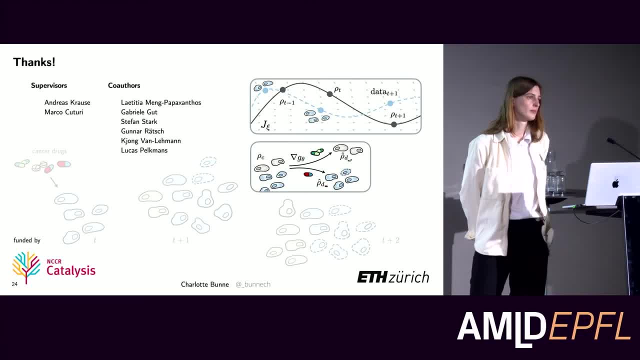 but also I've worked on biological problems and I've often come across the fact that biological processes are not optimal in many cases. Some features, for example cell shape, might be more tending to optimal states than, for example, gene expression or other metabolite expressions. 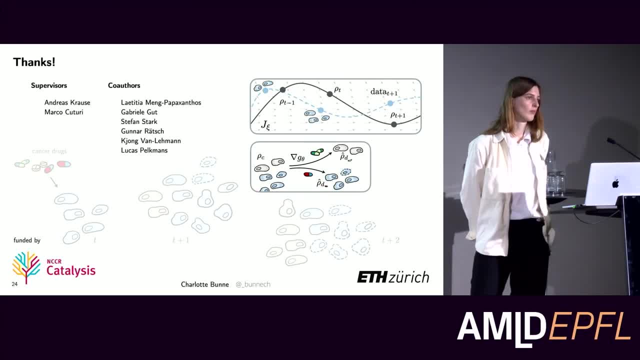 So my first question is: you know what are the cellular factors that your method applies more compared to others? And a very related question is, for example, gene expression-type data has different characteristics. For example, they often have Poissonian noise. 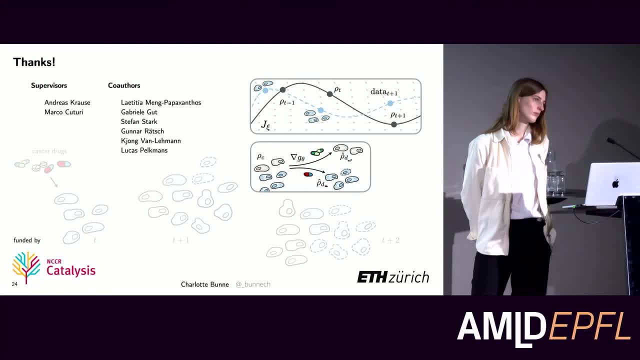 and other cellular parameters. Other cellular processes have, for example, Gaussian noise. So, in terms of stochasticity, are there different classes of processes where your method applies more than others? Yes, So maybe answering the second part of the question first. 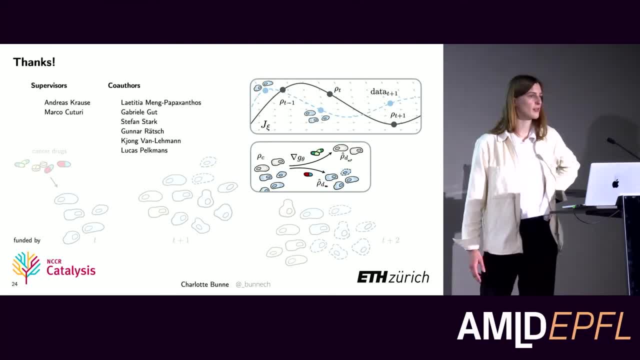 is so far, we have no assumption on the noise model, right, So we make no assumption of what kind of noise is in this data or in these processes. I have also rather recent work which somehow models these processes with stochastic difference equations. 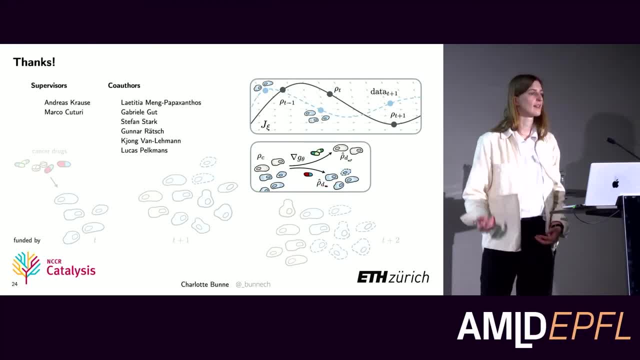 And I mean there you actually have the option of like adding this prior knowledge, you know about the process, into your update sheet, like into your stochastic difference equation. And for the first part of the talk, I mean all I can say: I'm not a biologist myself. 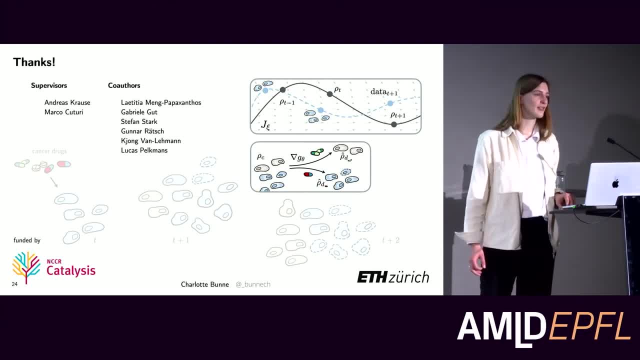 all, I can say that the data set I have received are of very different nature, So we looked at different data modalities, one of them being microscopy-based images, where we have morphological features as well as like certain like light sensitivities. 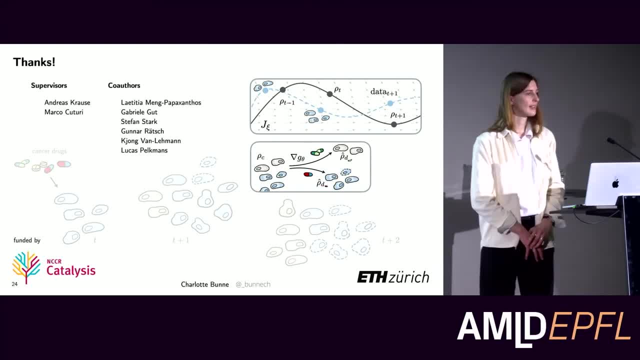 or detection of like signaling via certain markers, And so far this optimal transport hypothesis has worked very well for either like, for both morphology features, signaling features, but also for genomics data. I think the crucial limitation, but this is also something we address in the SELOT. 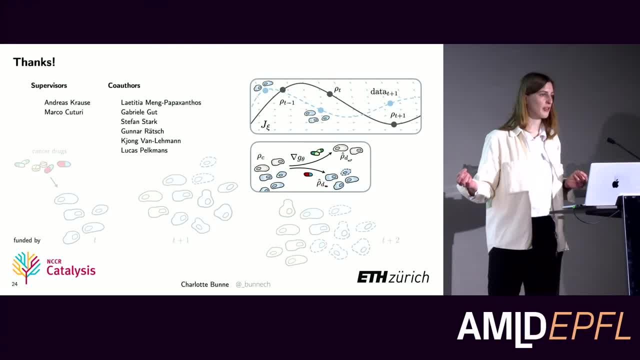 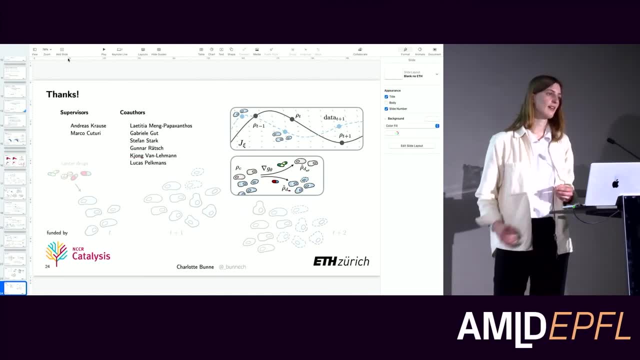 is that if you look at genomics data and you measure 5,000 genes, we still rely on a cost function of this optimal transport And, of course, here an L2 function like the L2 cost function in 5,000 genes. 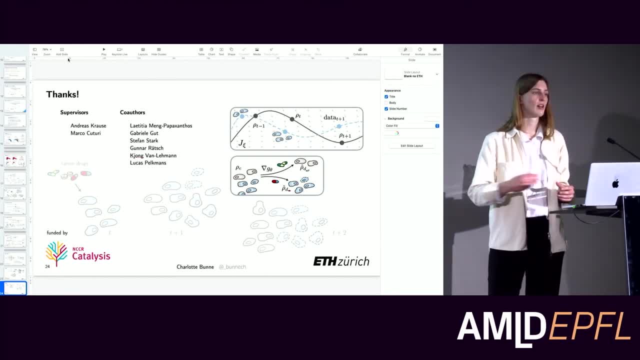 doesn't really make sense anymore. So then you need to actually find a meaningful low-dimensional embedding where you can then apply the optimal transport hypothesis. But still, even this like even if you need to find an artificial, like a low-dimensional embedding- 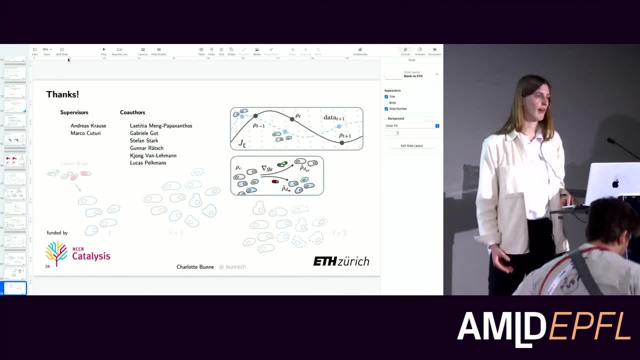 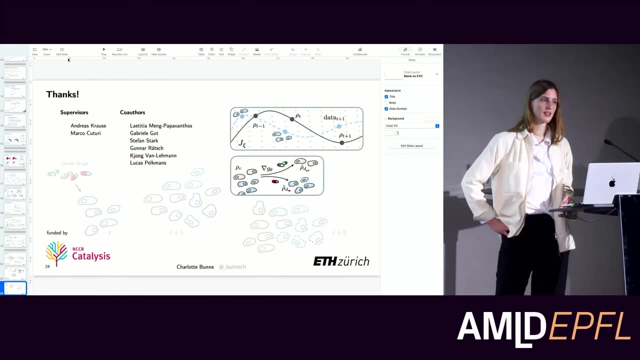 for our data and then apply the optimal transport. so far, we have really received very promising results, having the strong modeling prior in our data, in our model. yes, Okay, thanks a lot. Are there other questions? Thank you very much for the talk.